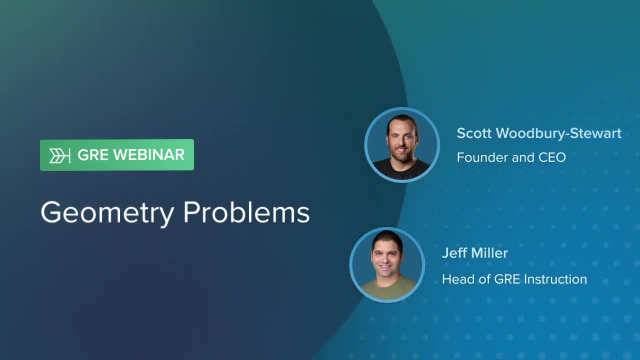 you're thinking of possibly switching. that is an option. If you know anyone who's taking a GRE, certainly let them know. I'll put the link into the chat. But it's super exciting, We're happy to have it and we're looking forward to it being equally as successful. 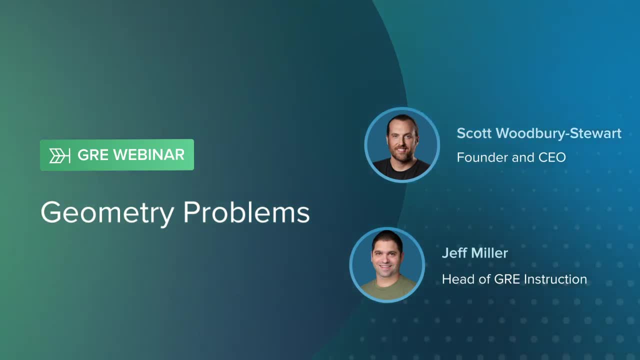 as what we've done with the GMAT. So, with that said, I want to get into the first question. For those of you who have been here before, you know the drill: I'm going to be giving questions. I'll give everyone. 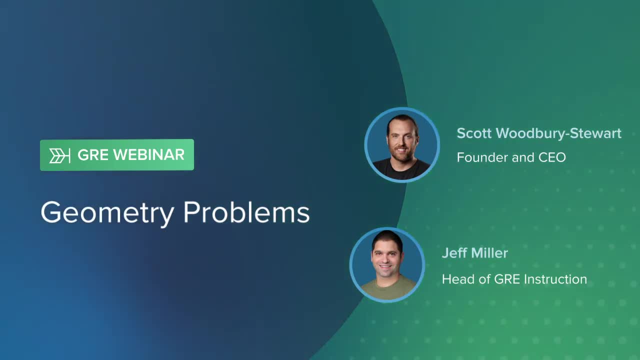 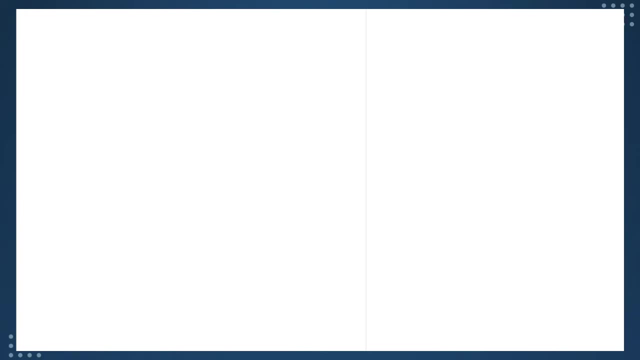 a few minutes to answer the questions And then, when you're done, you can put the questions in the- or your answer, rather in the- chat box, And from there I'll go to see what everyone's getting and then we will look at the solution. So the first question I want to do is a pretty 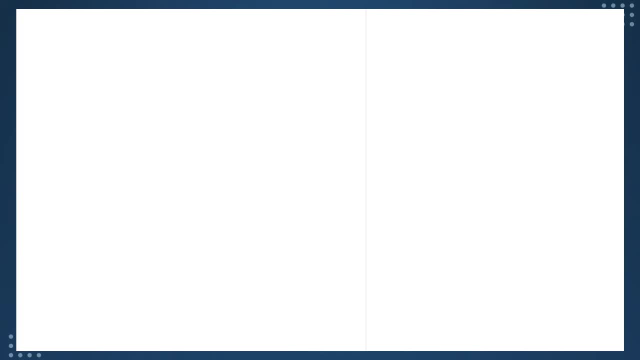 cool question. It's a question of testing you on, really, lines versus angles and triangles, And this is a type of question that they can throw at you in many different ways, But this is one very interesting particular way in which you can see it. So again, give everyone about. 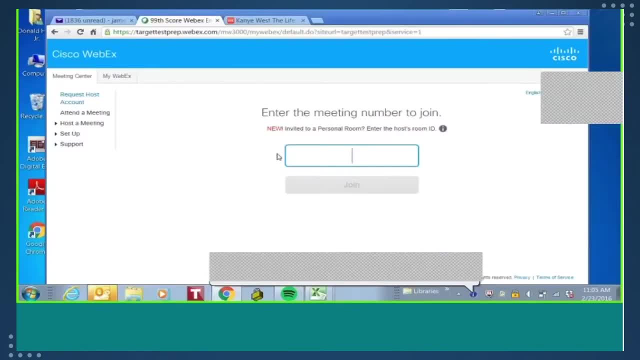 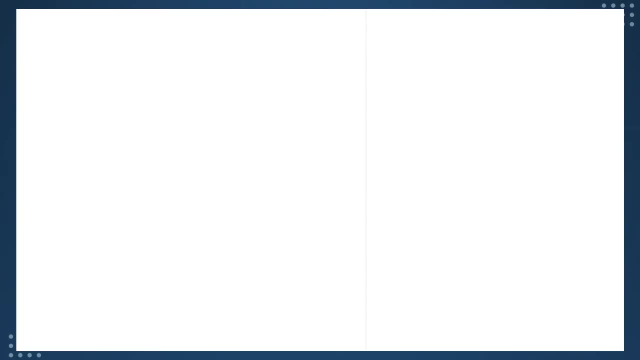 two minutes and then chat about the result. I'm not sure why some of you didn't get it. Someone just stole a ball from me, but I stole a pen. Okay, There's the first question. everyone, As I said, put your answer in the chat box, so we know what's going on. 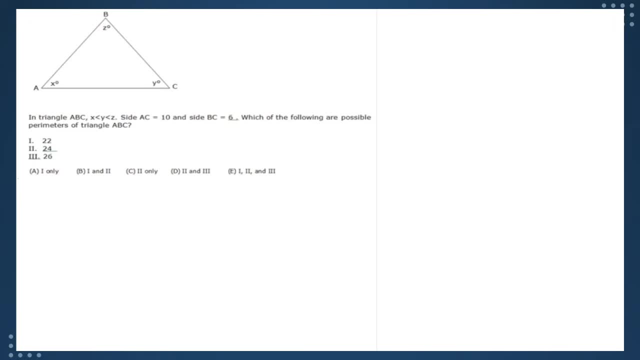 Okay. So the first question I want to ask you is: how do you know what's going on? So the first question is: how do you know what's going on? Okay, So the first question is: how do you know what's going on? 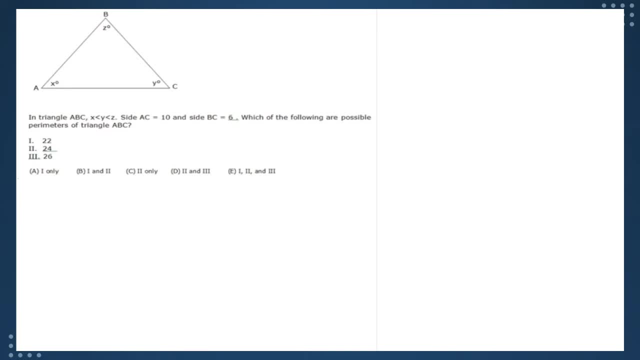 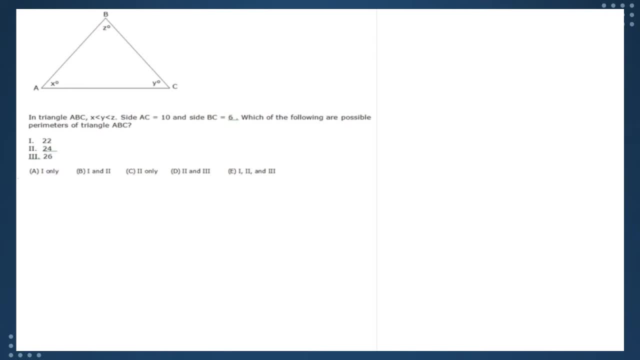 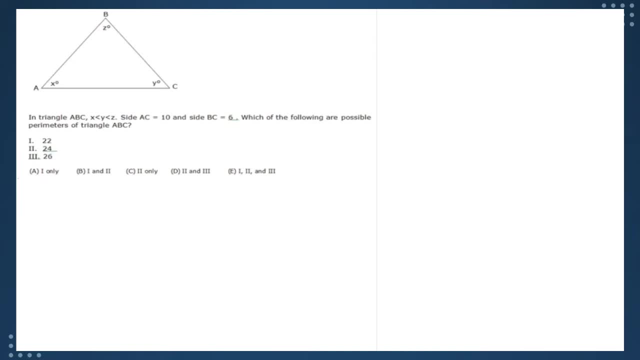 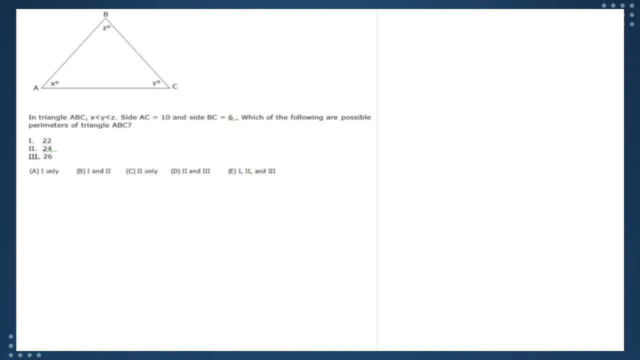 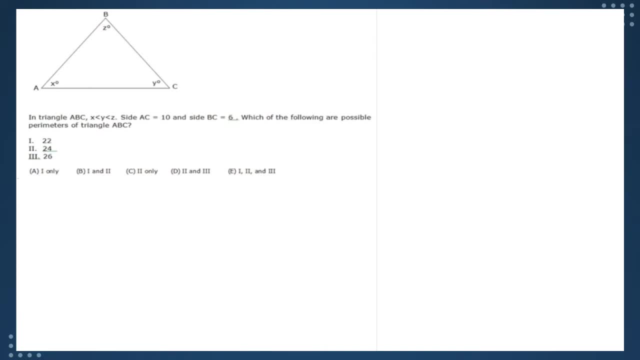 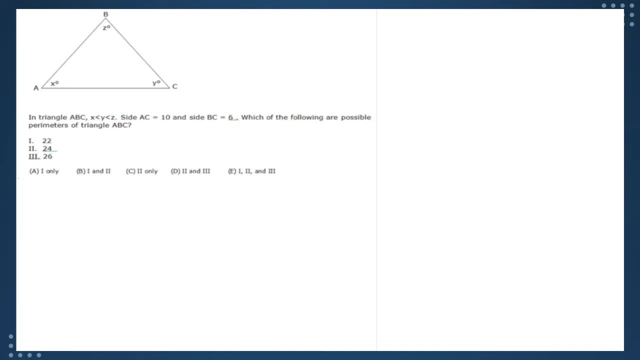 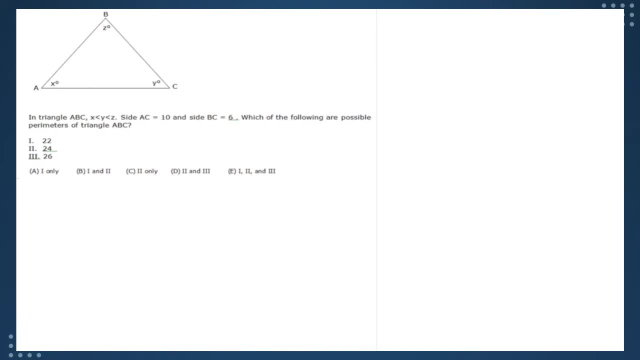 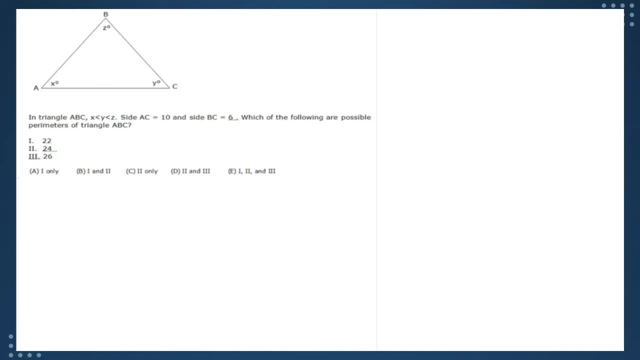 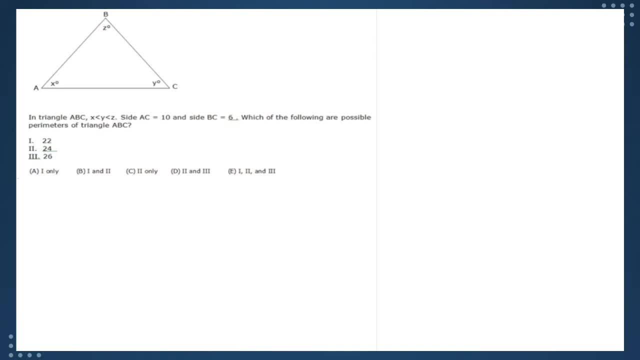 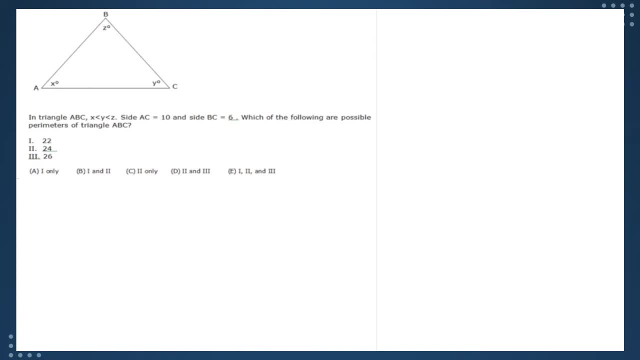 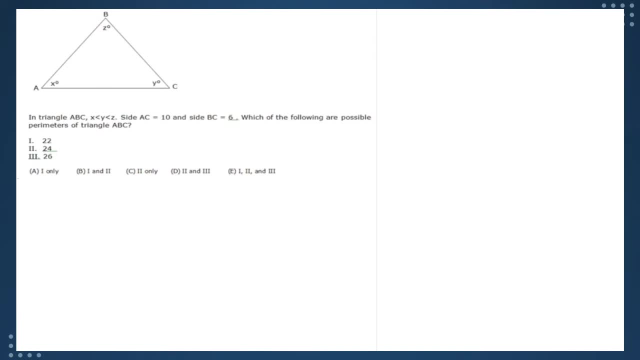 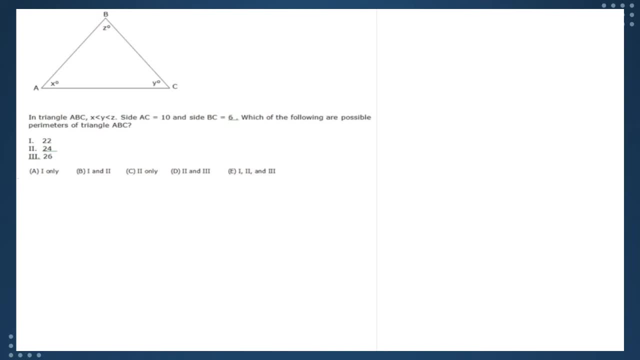 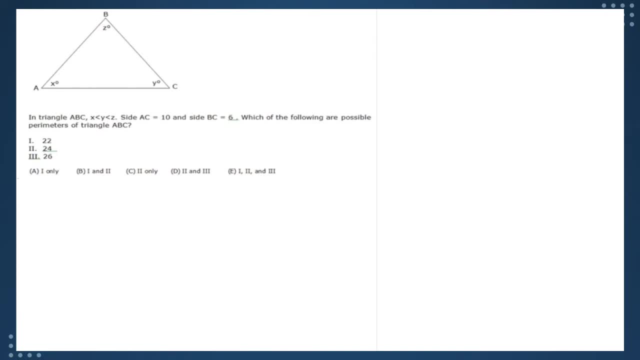 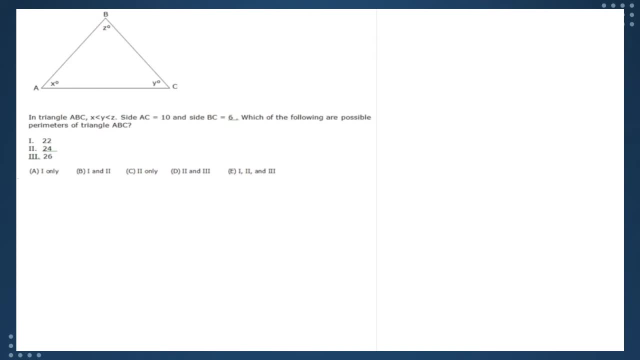 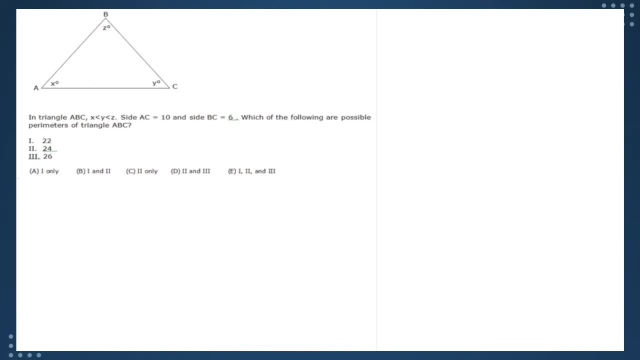 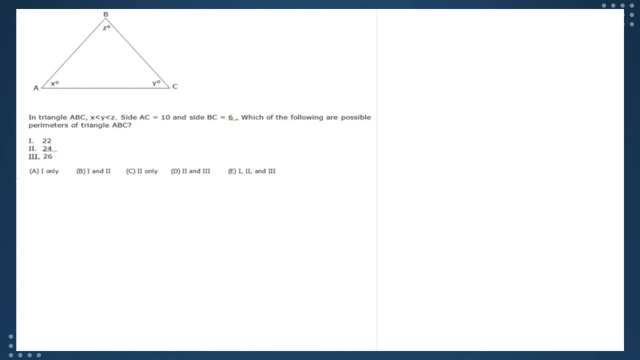 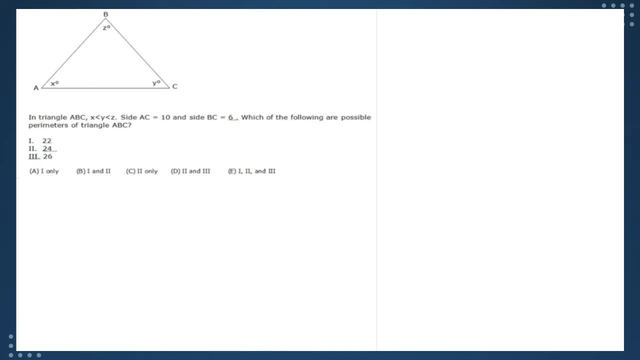 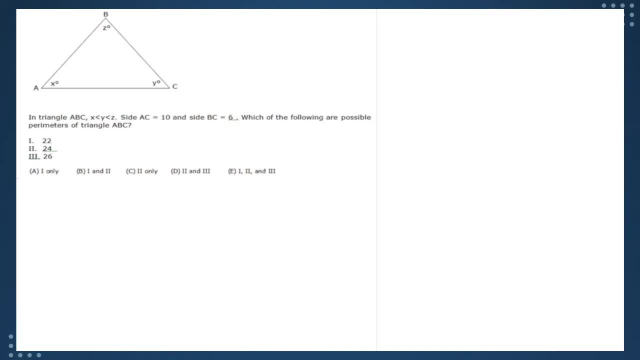 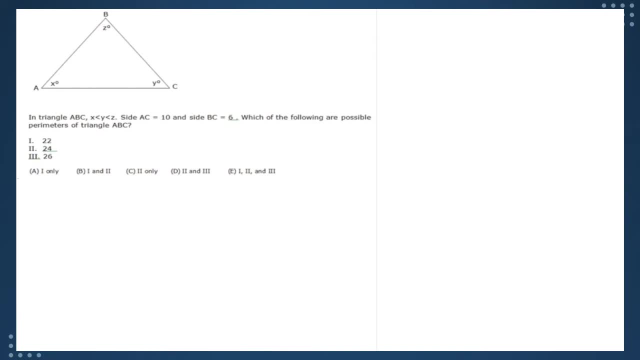 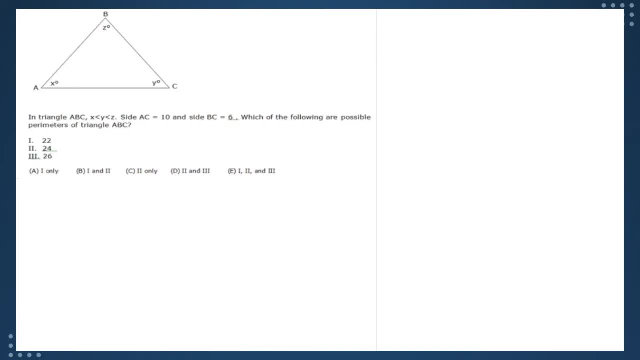 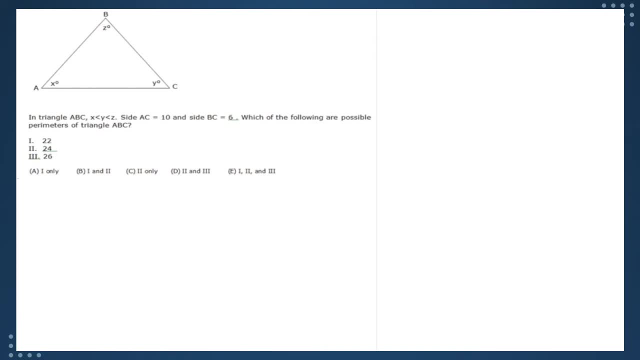 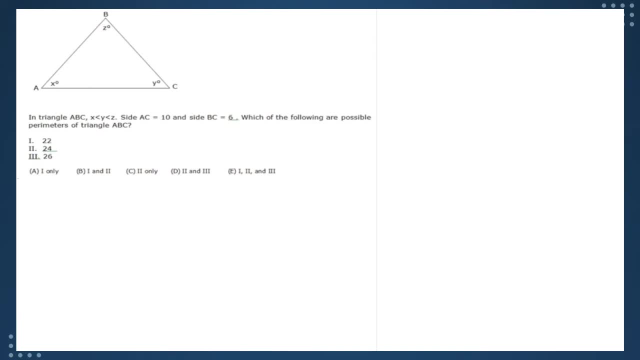 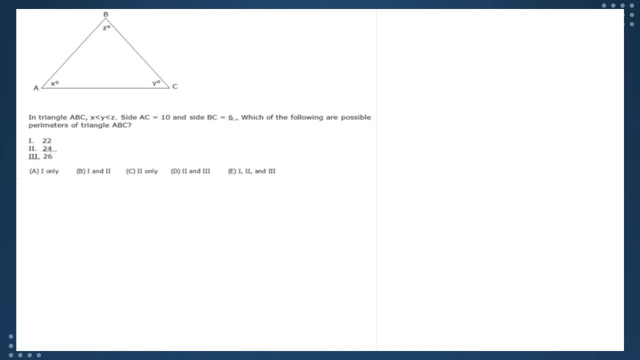 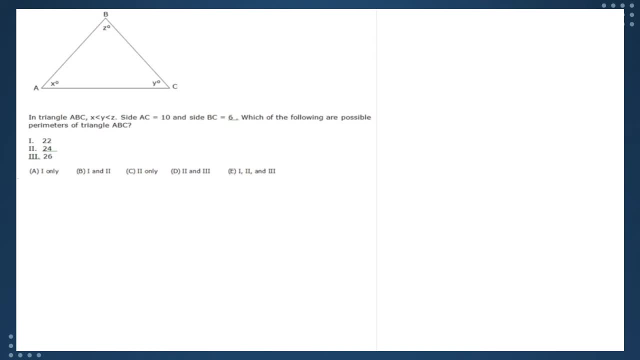 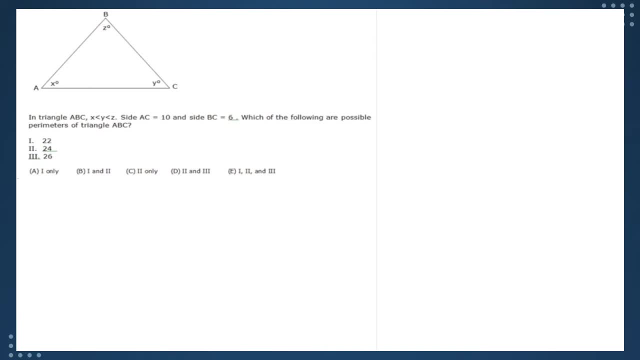 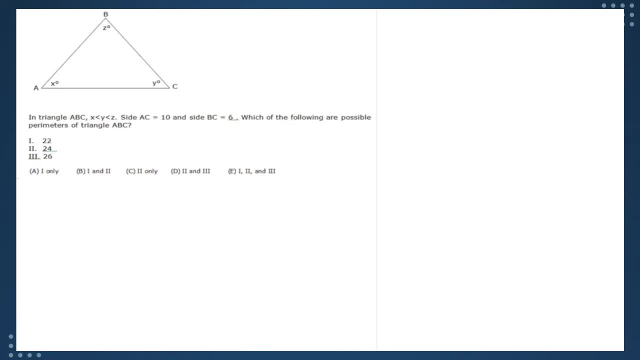 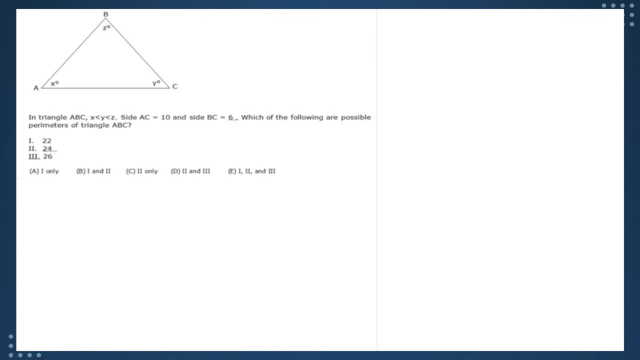 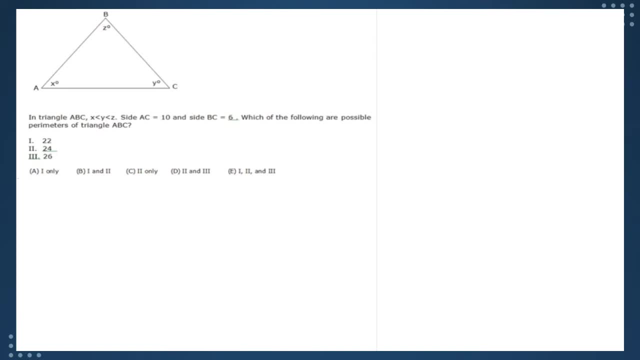 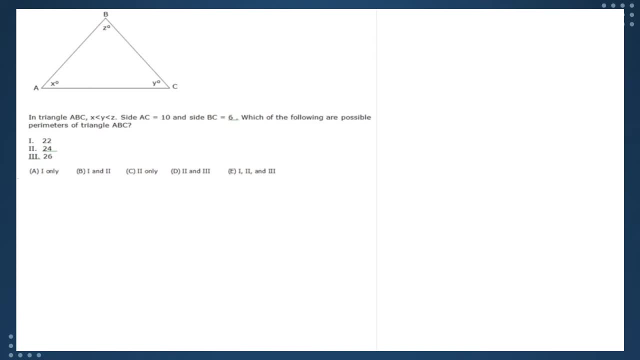 Okay, So the first question is: how do you know what's going on? So that was roughly two minutes there. This is a great question, because one of the things with triangles is that the angles of a particular triangle correspond to a particular side of a triangle. 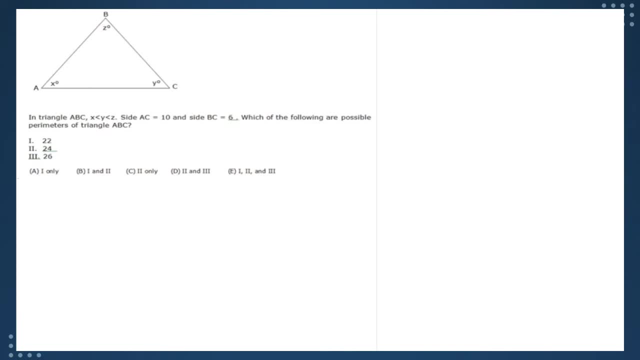 So, to be a little bit more detailed about what I'm saying is, in this problem we are given that X is the smallest angle in this triangle, which means that BC has to be the smallest side. We're also given that Y is the middle angle, which means this has to be- for lack of a better word- the middle side. 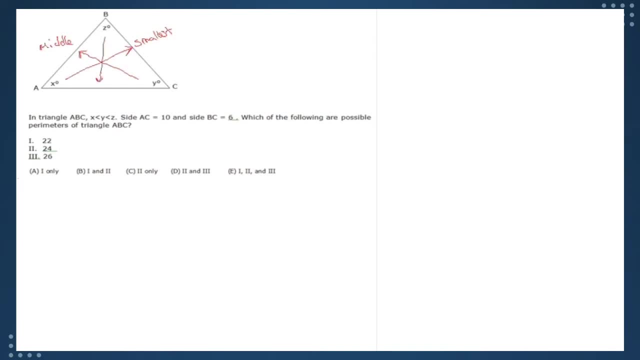 As far as length, And then this has to be the largest side. So the minute that we know that AC is 10, and the minute that we know which corresponds to the largest or is the largest side, and the minute that we know AC is- excuse me, BC is actually 6,. the minute we know BC is 6,. 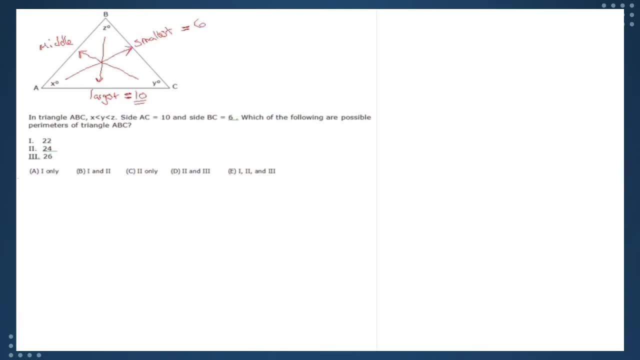 we know that the middle side has to be Between 6 and 10.. Now we're not told that the sides have to be integers, but we can see our answer choices are in integer form. So the possible middle side is between, and we'll just call M for the middle. 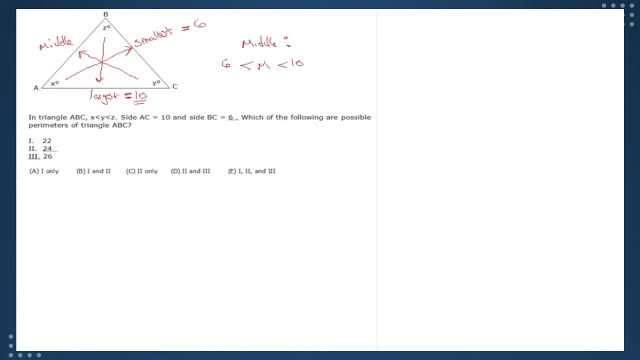 is going to be greater than 6 and less than 10, based on these angle measurements. So that gives us possible options. Now, If we take the 10 and 6, that's going to give us a total of 16.. 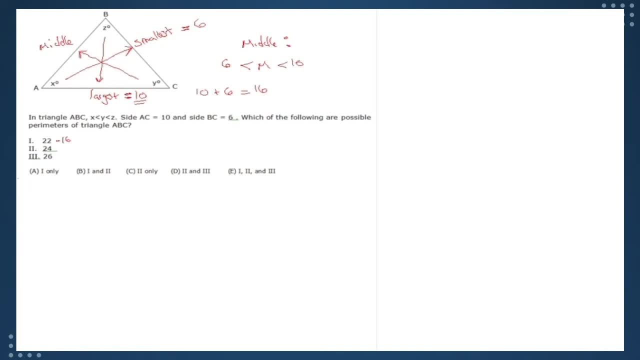 So if we subtract 16 from each one of these Roman numerals, we get a possibility of 6,, we get a possibility of 8, and we get a possibility of 10 for the middle side, And what we can see is, since M must be between 6 and 10,, the only logical option here is 8,. 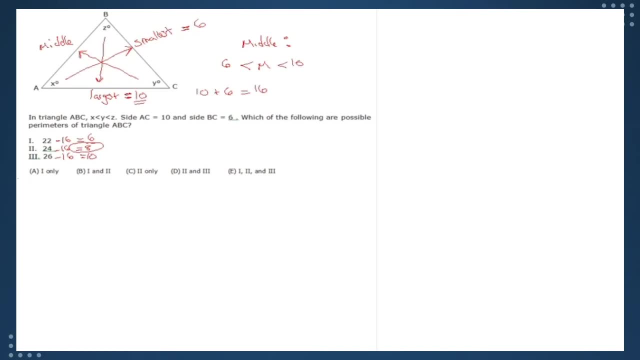 that corresponds with number 2, and that is the answer choice. So they can test this in a variety of ways. you know, be prepared to see it in a variety of ways on this exam, but you know this is like anything else and I say this every week, that you know. 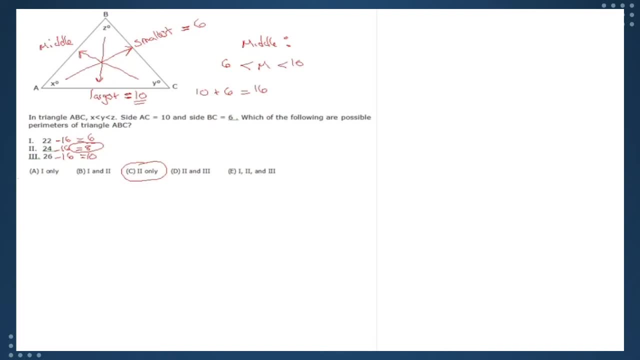 we're in a situation where, if you know these small rules, you're going to get to a question like this and you're going to immediately have a process. You're going to have a process of how to deal with it. The flip side is, if you don't know these rules, you get to a question like this: 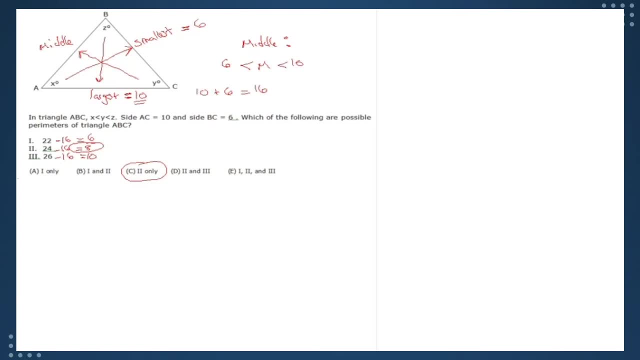 and let's say, you don't have a process immediately of how to solve it. So what I want to do next here, just getting in another question, is I want to do another interesting problem that deals with triangles. Sometimes you're going to they're going to try to trick you on where the height is of a particular triangle. 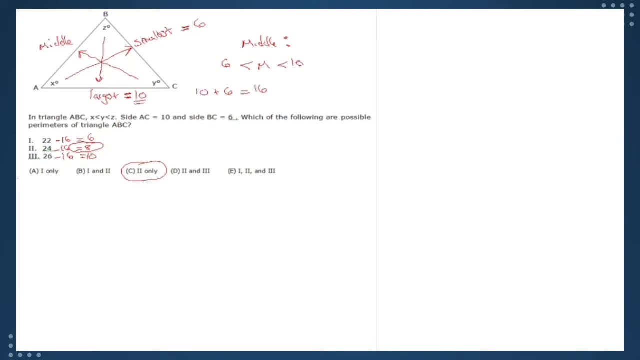 Now I wouldn't say that this problem is the hardest- It's not the hardest problem in the world- but I would say that there's definitely some ways in which they're trying to trick you or trap you here into thinking you know. 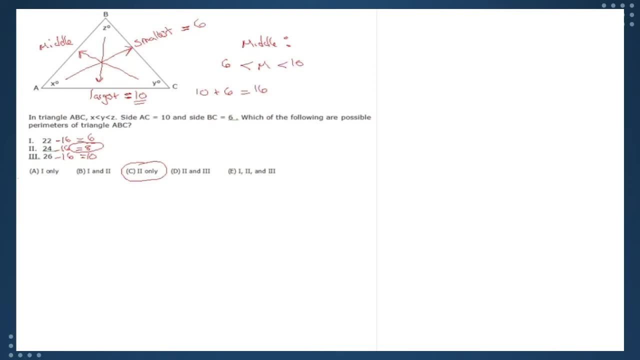 what the height actually is of the triangle. So when everyone's going through this question, do a really good job of making sure that you're finding the height versus the base and stuff like that. There's a lot we can talk about once we go through this question. 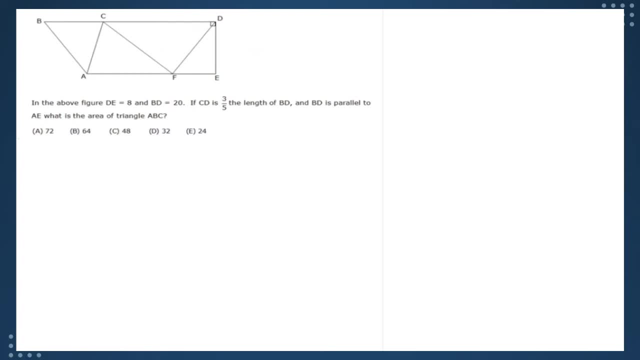 So I'll give everyone about two minutes and then we can go from there. All right, All right, Thank you, You, You. Okay, let's get after this one here. I do see a lot of correct answers here, which is good to see. 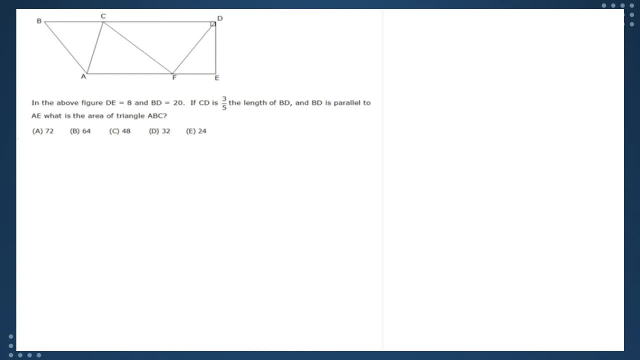 So what's kind of going on in this question Is the idea of where to find height in a particular triangle, and one of the things to understand is the height Really in any polygon for that matter, but it's more kind of Front and center within triangles- is the height has to be perpendicular to the base. 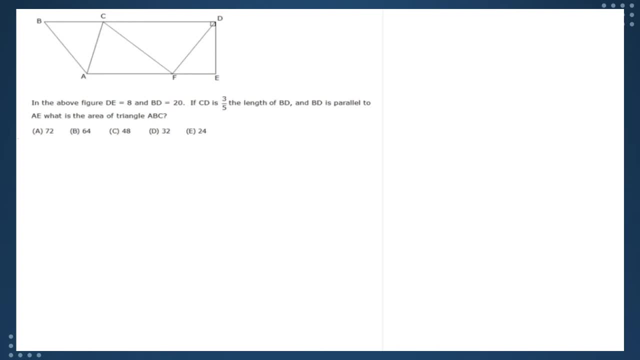 We just take that for granted. when we look at, say, a rectangle, because you know The width is perpendicular to the width or the length. or if you look at a square, The side is perpendicular to the side, You never really Actually have to think about it, the triangle. these exams are forcing you to think about it. 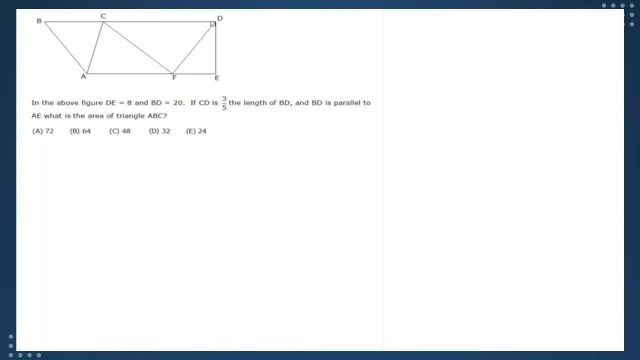 So in this particular instance, first and foremost, there's a lot of information. We need to fill that in. so we have de is a. We have BD as on whole Is 20. We have CD is 3 fifths of 20. so 20 times 3 over 5. 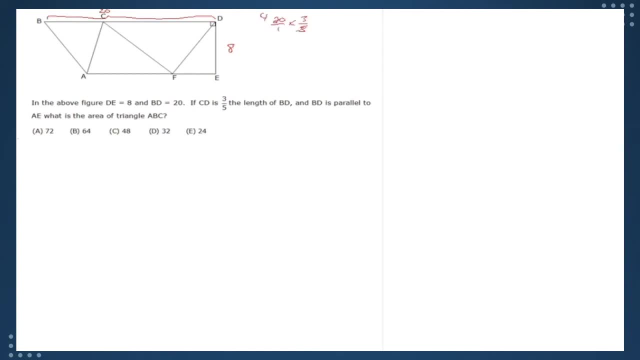 and gives you 12. So if CD is 12, I'll change the color. means BC is A. Now the question is saying B. that was telling us that BD is parallel to AE, which is important and we need to know what. 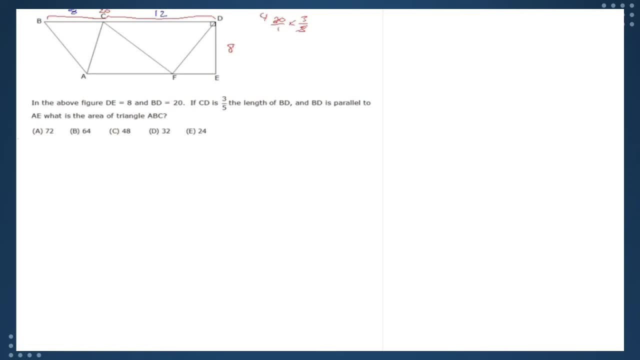 the triangle is of ABC, so we need to know the area of this triangle. here Now, the interesting part is that the height is not AC. Some people may think it is. they may be trapped to think it is. they may think BA is the height. 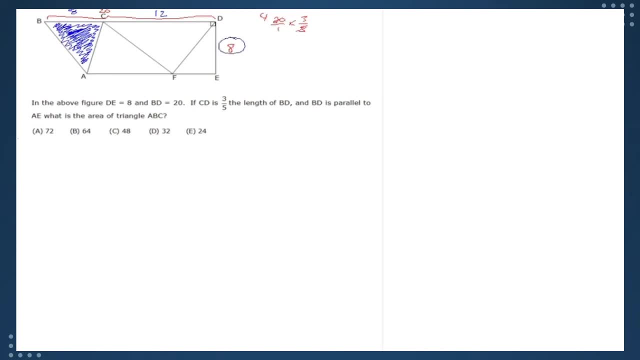 but really the height is DE and if you were to basically slide this over, this is the equivalent of DE and that's going to be A and that's also the height of this triangle. So the height I mean. another way to look at it too- is if the height can be or change. 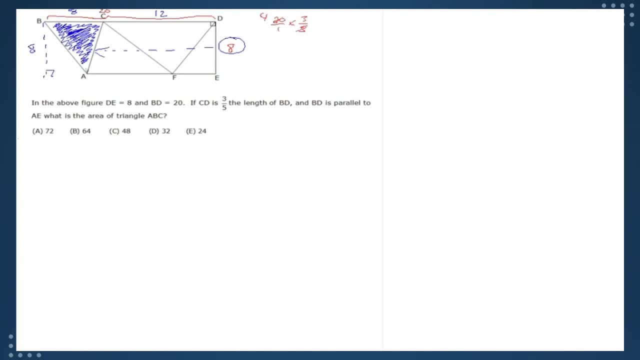 the color, the height can effectively be here, but it doesn't really matter. The point of this question is that the height doesn't necessarily have to, It doesn't have to touch the triangle that it's the height of, it simply has to represent. 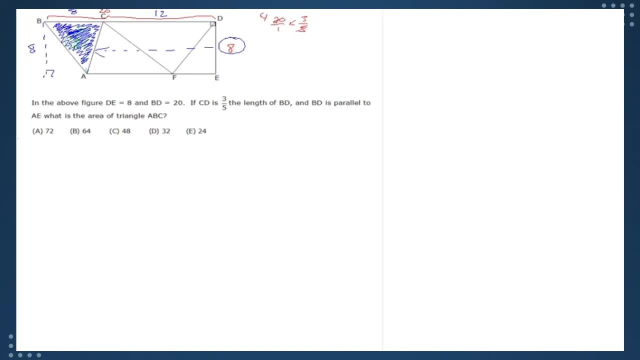 it. So if we see that the height is 8, and the base is 8,, since the area is 1 half base times height, we have 1 half times 8 times 8,. the answer here is 32.. So it doesn't look like too many people fell for that trap there, which I'm happy to see. 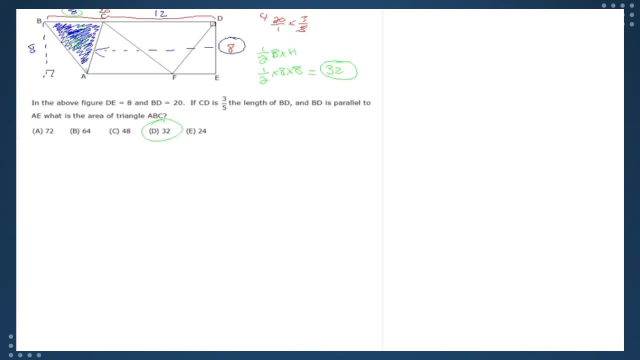 I do want to get into one other type of problem, another rule that I'm not going to use, but I'm going to. well, actually, let's hold off on that. I want to get into some extract shapes, since we have about 25 minutes. 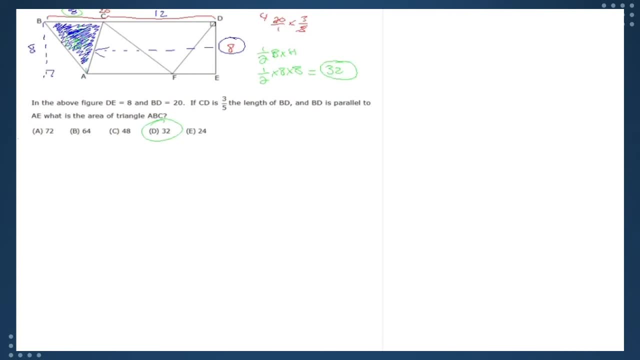 So what we're going to move on to doing here is we're going to start off with circles, central angles, how those work, and then I want to deal with triangles. inside circles, There's a lot of inscribed shapes that are asked about on the exam. 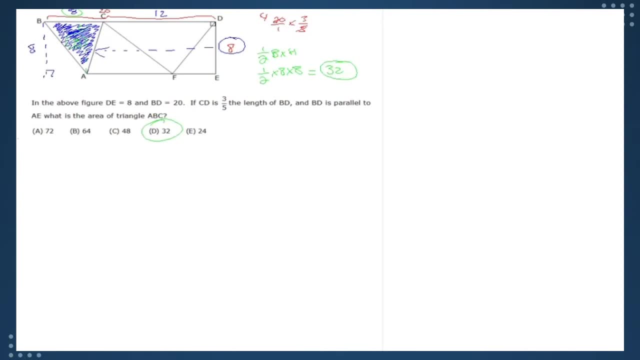 One of the most popular, in my opinion, that you'll see a lot of has to do with triangles inside of circles. I've seen on this test, But before we even get there they do like to test a lot on central angles and things. 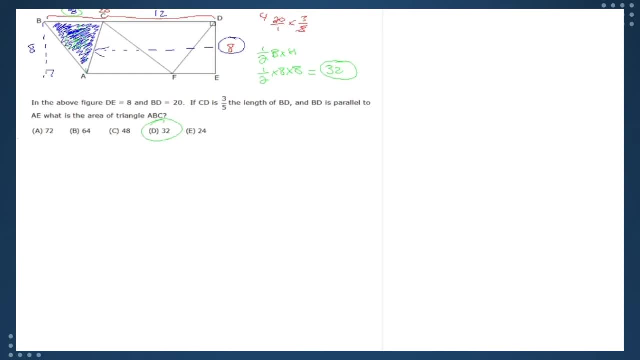 like that within circles. So I want to talk about central angles and how they relate to arc length, and I want to talk about central angles and how they relate to area. So the first question we're going to do is here: Give everyone a few minutes and then we can chat. 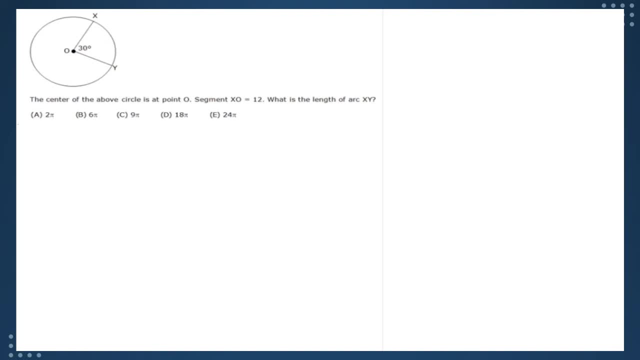 We'll be starting in about a minute, Okay, So there's a lot of stuff that we've discussed, that we brought up. that's already a big issue with this. I'm just going to chime in, put: they've been bringing anything up together. 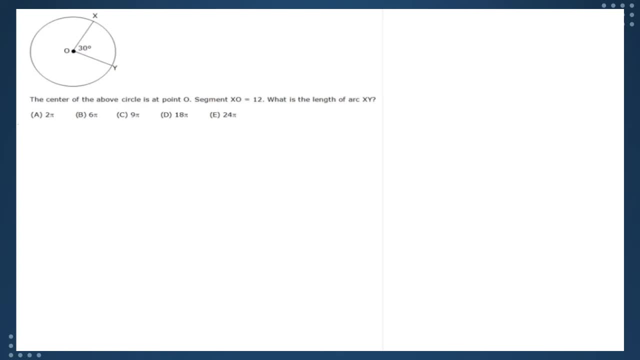 So take a look at that. We're doing some conflicts, you, you, you, you, you. okay, so this is test thing um. a very interesting rule here, and what that rule is has to do with um: how a central angle in a circle is proportional with the arc. 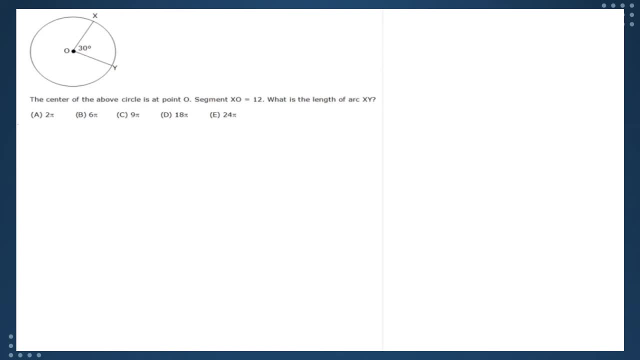 length. so what you'll notice here is it's saying the center of the circle is at point O, which means this 30 degree angle here is considered the central angle. so there's a really great proportion um that exists um anytime you have a central angle within a 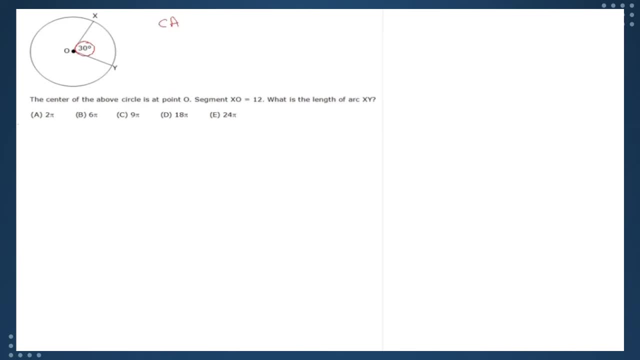 circle. so you can say that the central angle, which I'll label CA, is 2360 as the arc length. and when we say arc length that just means a kind of fractional component of the um. circumference is to the circumference. so again, so central angle is 360. 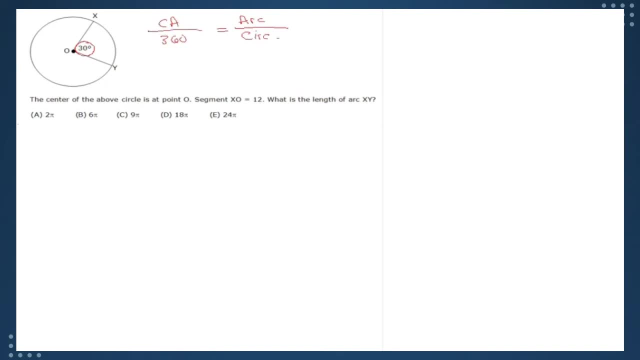 as arc length, all very important stuff for now. now we have to actually fill in our values. so we know what the central angle is- it's 30. we know that the total degree measurement is 360. we don't know the arc length, which is obvious because it's. 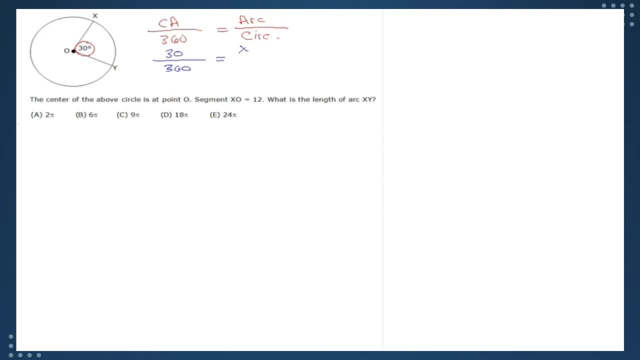 a little too far and we have to determine the circumference, since segment XO is 12, we see that. that's the radius. remember circumference is 2 pi r, so circumference is 24 pi. that, and then that. now, one of the things I always say to do. 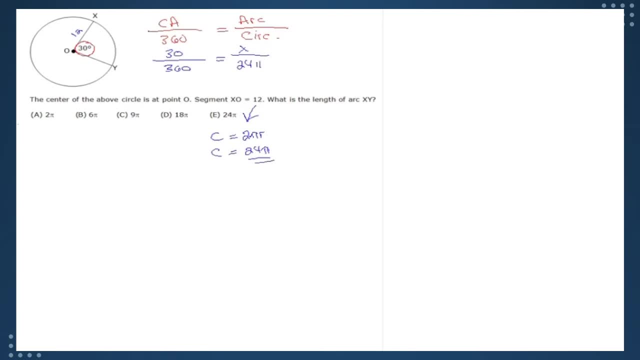 and it doesn't matter. you know, um, you know where you're at in the test. you always want to look to reduce. you want to look to reduce the circumference, and that's what we're going to do. so you want the numbers to be as small as possible. 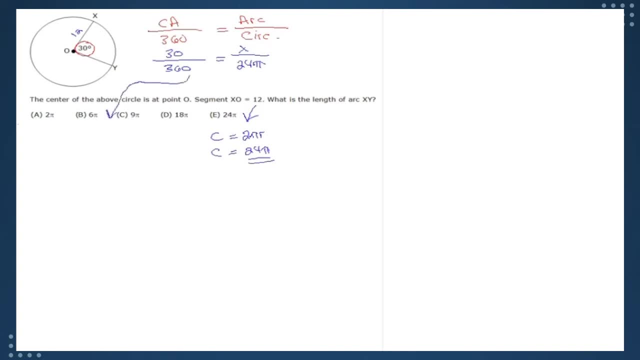 at all times. so 30 over 360 actually will reduce down to 1 over 12. so we can say: 1 over 12 equals X over 24 pi. cross multiply 24 pi equals 12 X, X equals 2 pi and there is. 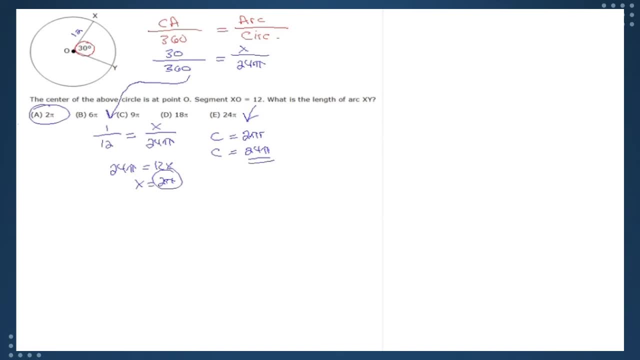 our answer. so this is a great thing to have tucked away everyone um central angles. you know they love to ask about them. there's a lot of kind of variations they can do with this stuff and remember this can also relate to when we have um inscribed. 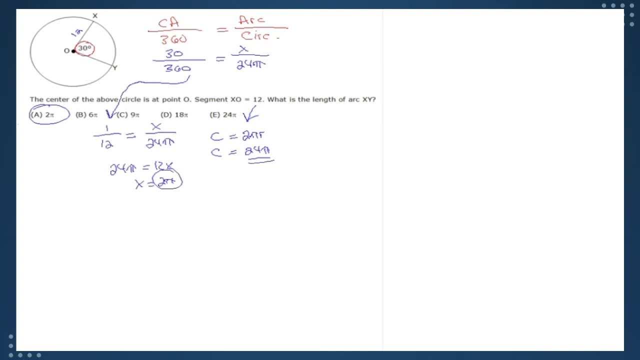 angles in these circles. right now we're really only talking about central angles, but as we get into inscribed shapes we'll start having to deal with inscribed angles. we're going to get to that, obviously. before we end, here's one other question I'm going 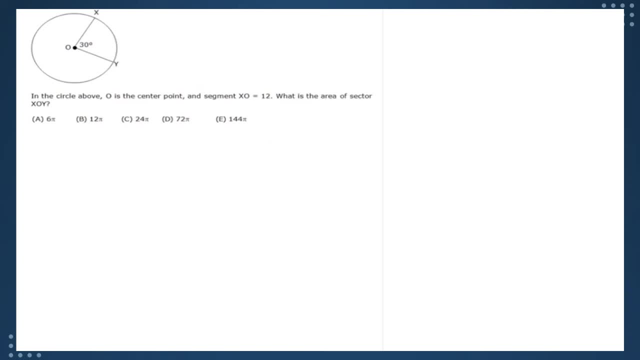 to do that deals with this. so now I will say what I was saying. again, this is going to be pretty much the same proportion that we use. the only difference is that this here is sector area, this here is total area. so this is going to be: 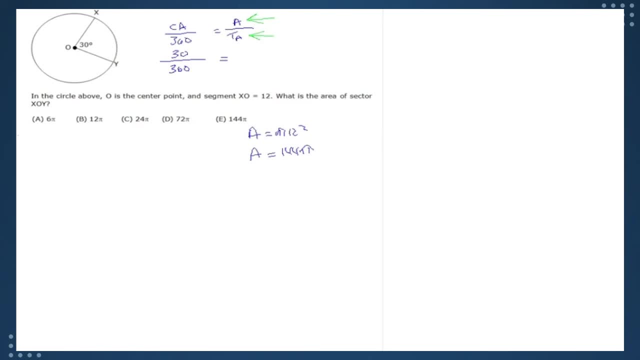 the only part of this problem, so we need to use it in different ways. for example, XO is still the radius, but to get the area we need to do PI R squared, so the area becomes 144 PI. so if we do this out in full, we see. 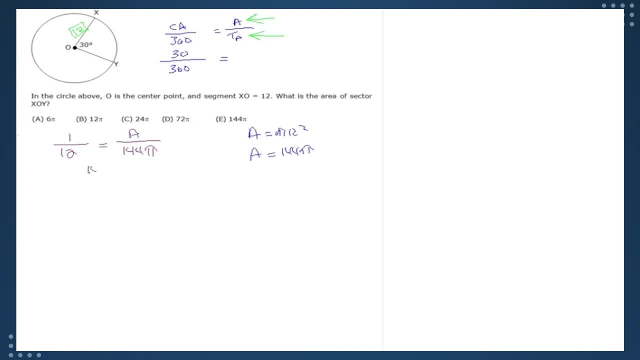 that we have. 1 over 12 is 144. PI equals 12A. divide everything by 12 and A equals 12 PI, and the answer here is B. so now we get to get into what I was talking about before, which is inscribed shapes. 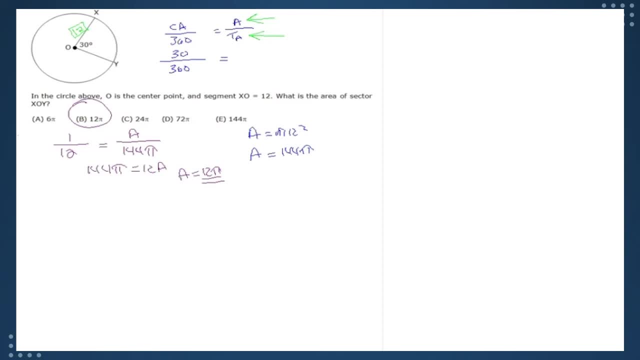 in circles. there are going to be some slight changes, cool things I can teach you about as far as relationships go, and one thing you can do is ask about the other shape, meaning there has to be some sort of shared side in order to be given information about. 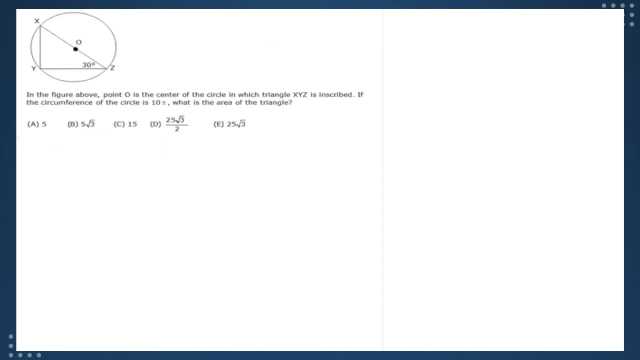 one shape and then ask about the other shape. now that might seem convoluted. obviously, I will explain myself further once everyone dives into this question here. so I am going to talk about some of the most important things that we need to talk about in this session. 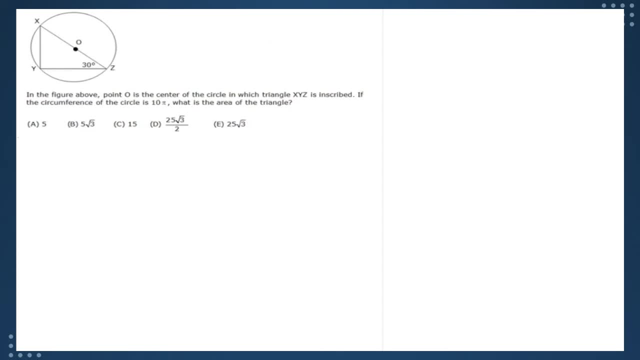 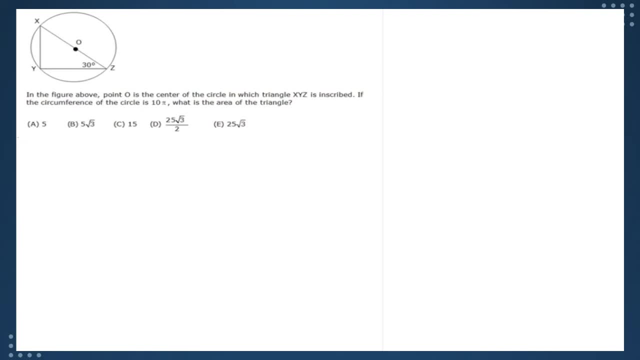 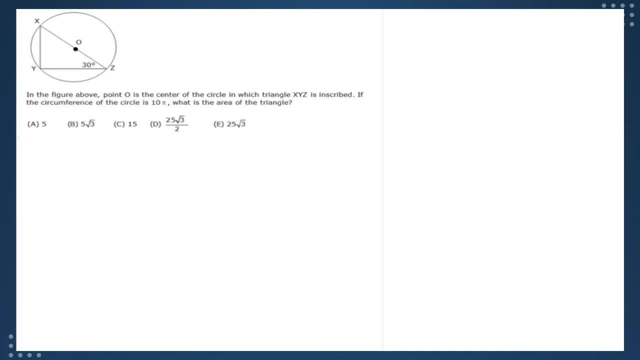 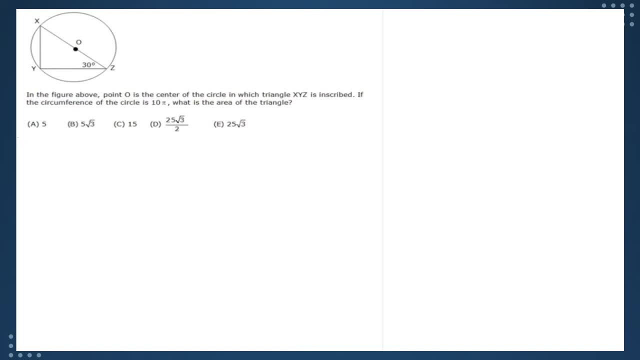 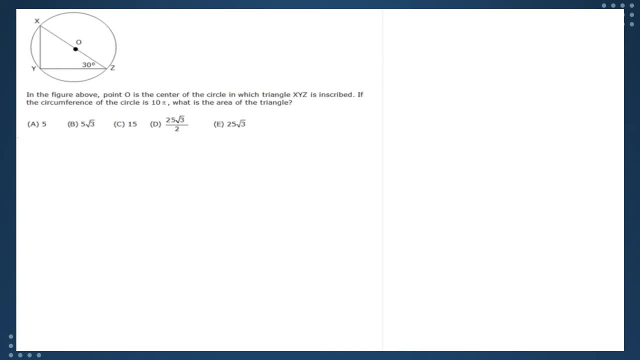 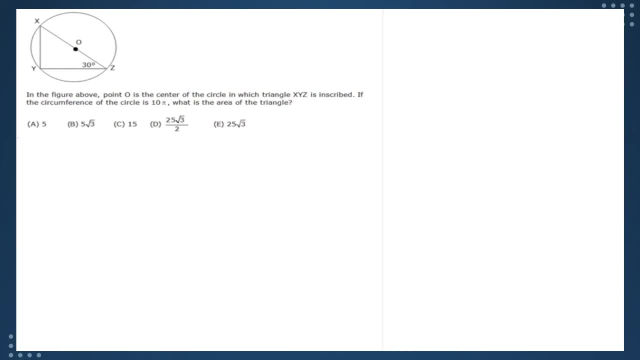 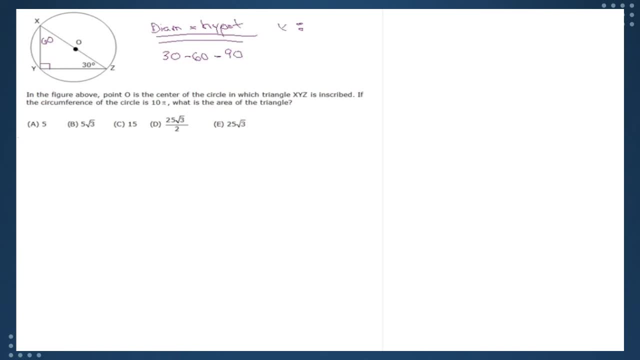 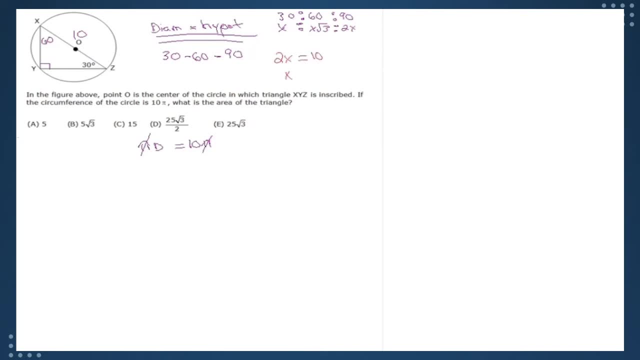 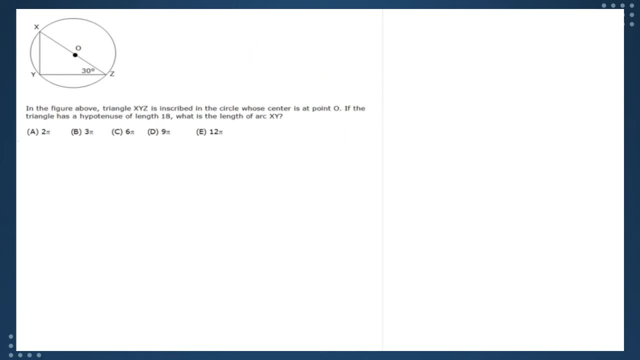 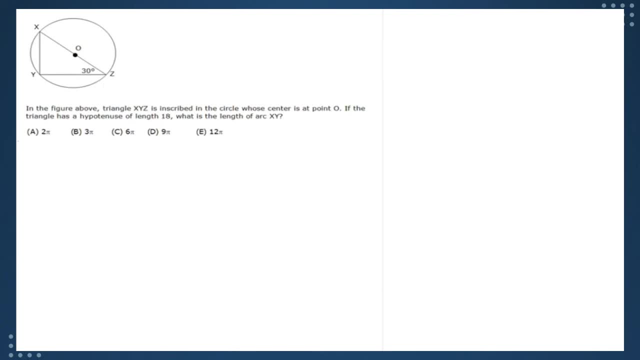 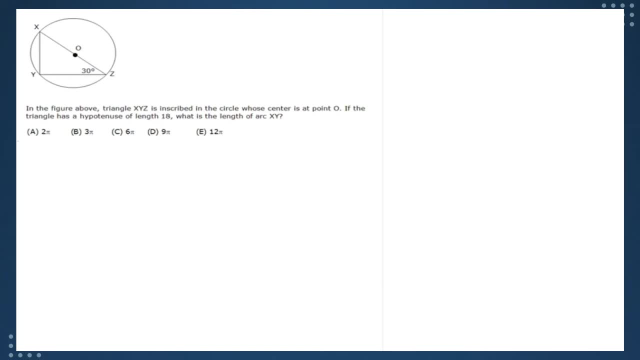 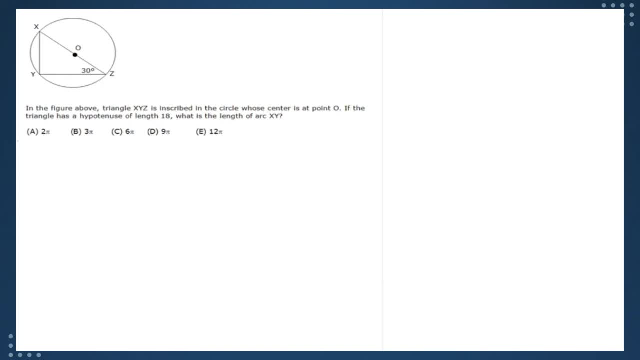 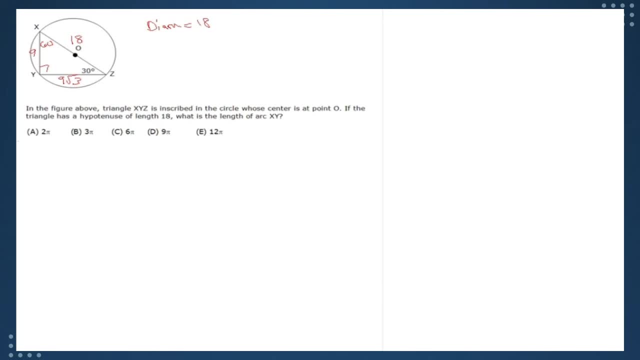 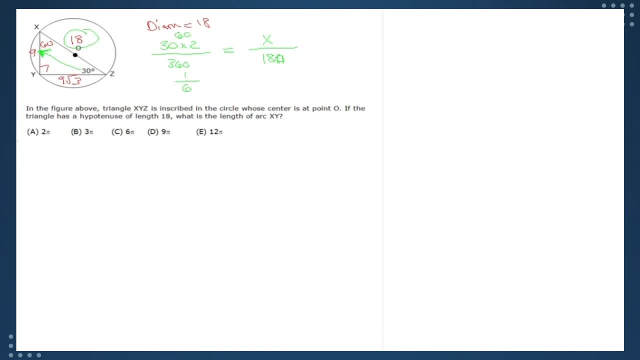 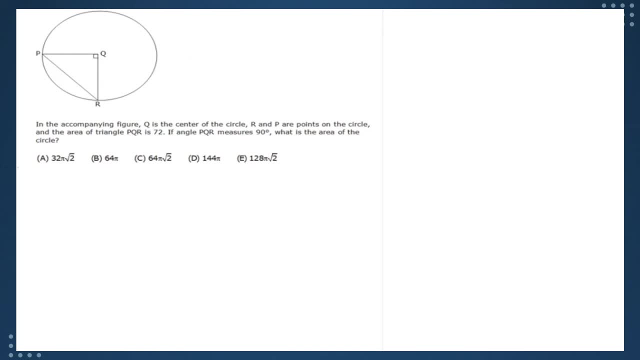 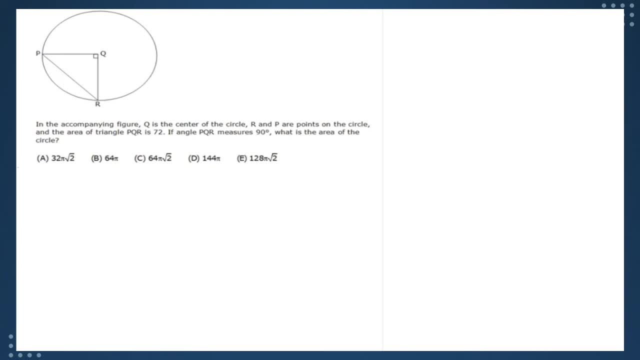